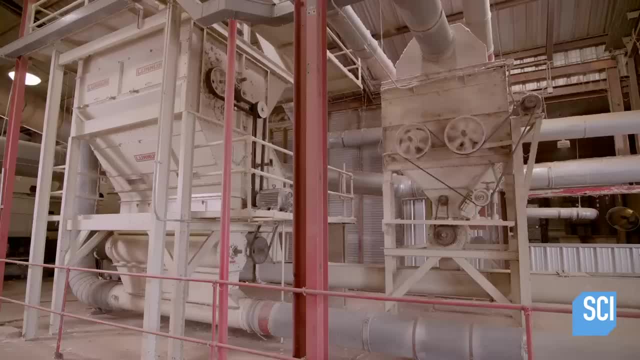 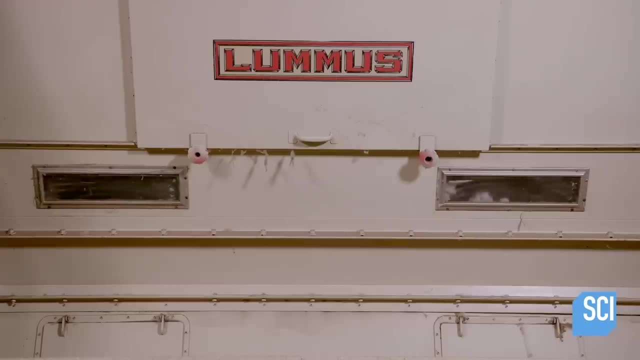 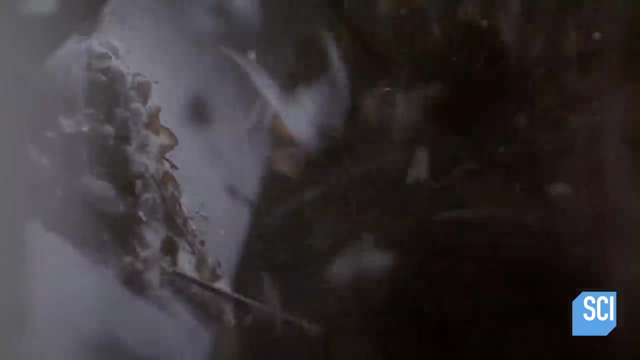 through a machine called the steady flow, which divides it equally between two processing lines. On each line, the seed cotton enters a burr machine which grabs the seed cotton with a circular saw and swings it against metal bars. The centrifugal force shakes off the heavier debris. 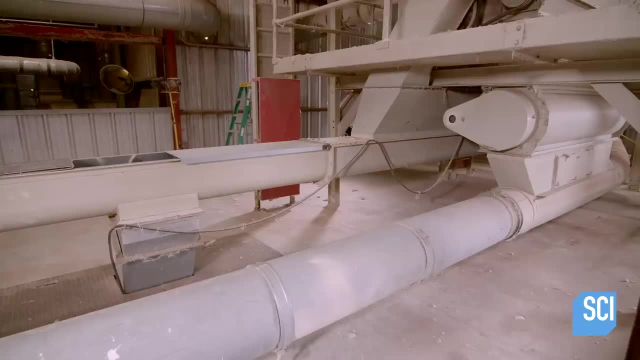 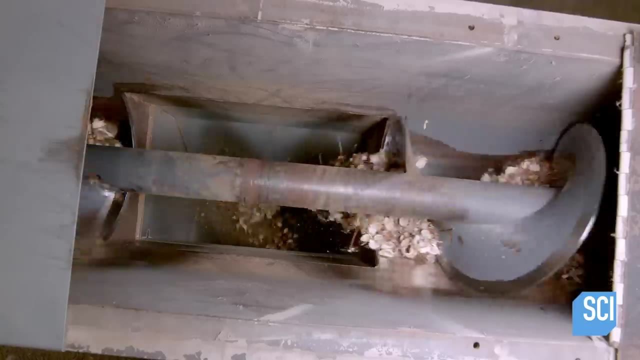 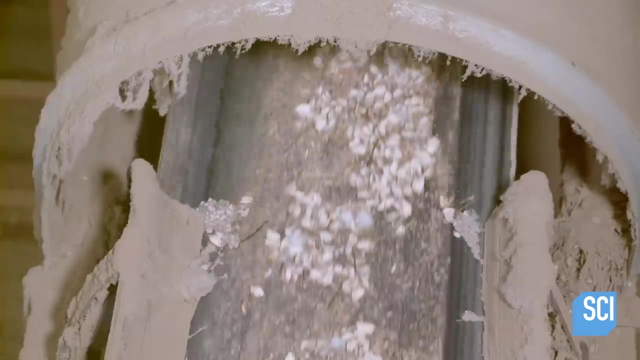 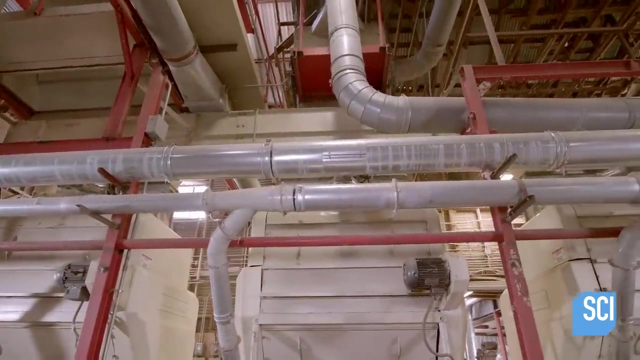 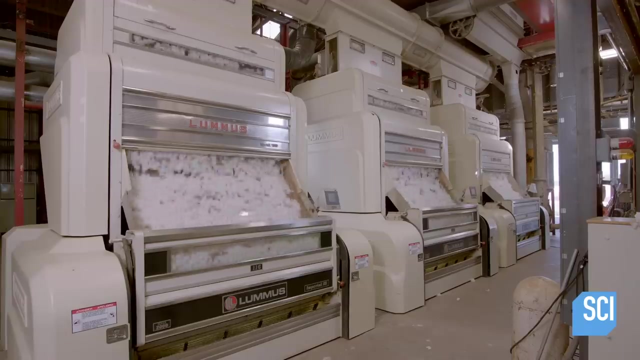 The seed cotton exits the machine through one pipe and the debris through another. A large auger transfers the debris to a waste chute and out of the plant. The seed cotton is ready for the final stage of processing. A network of pipes feeds a row of machines called gin stands. The gin stand separates the seed from the fluffy stuff. 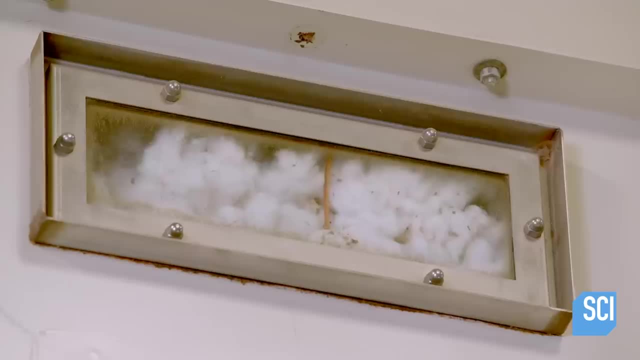 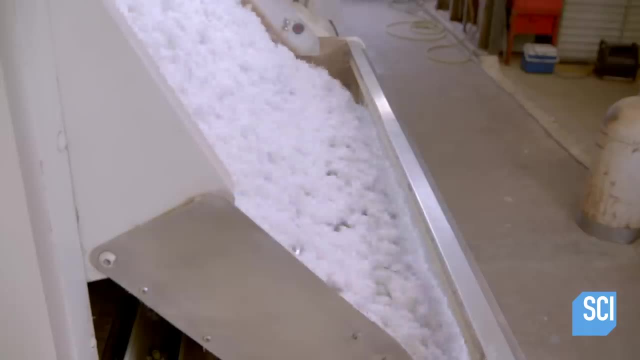 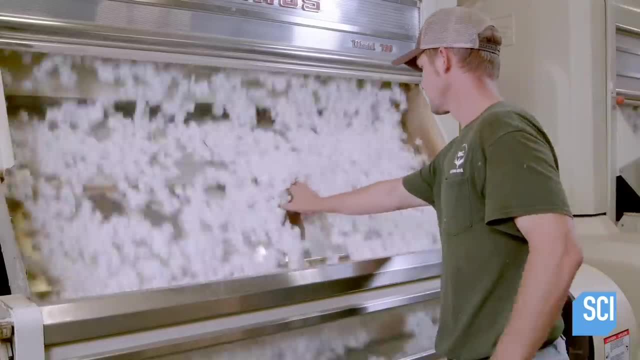 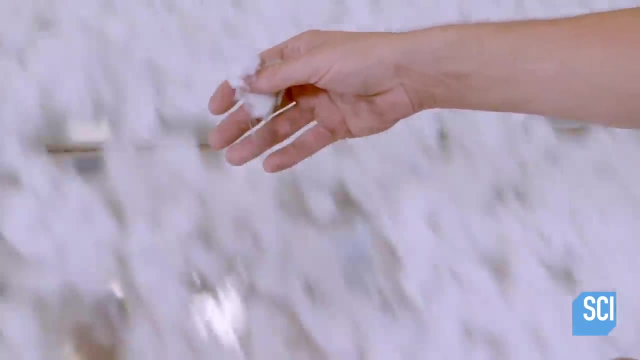 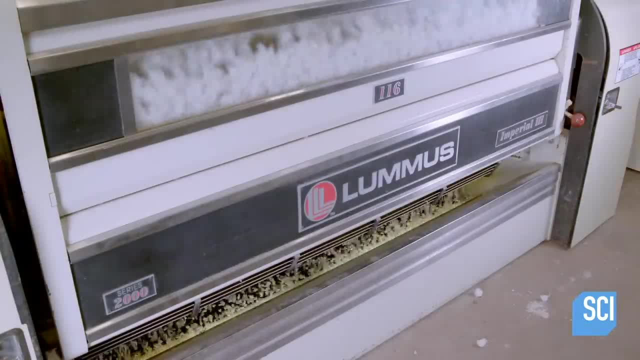 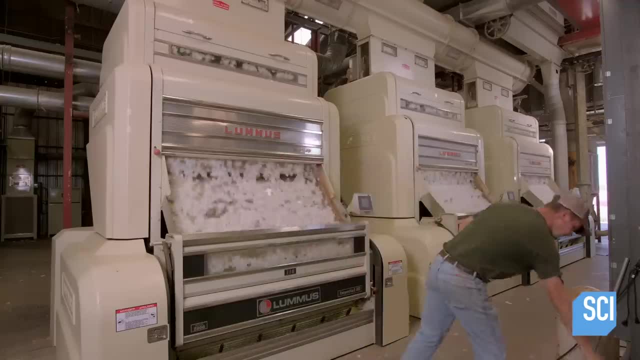 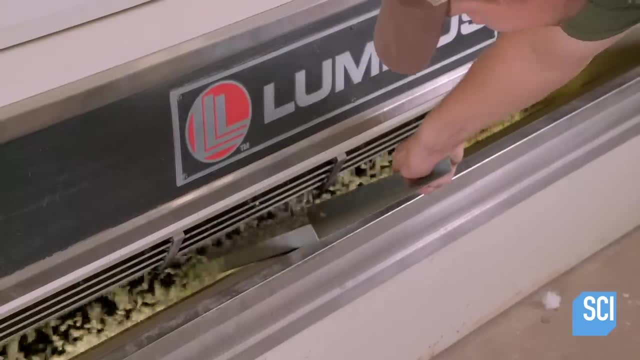 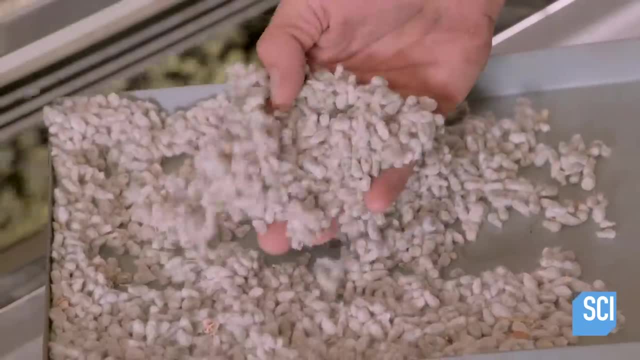 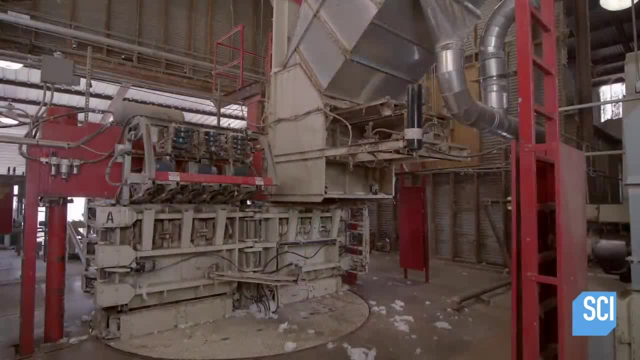 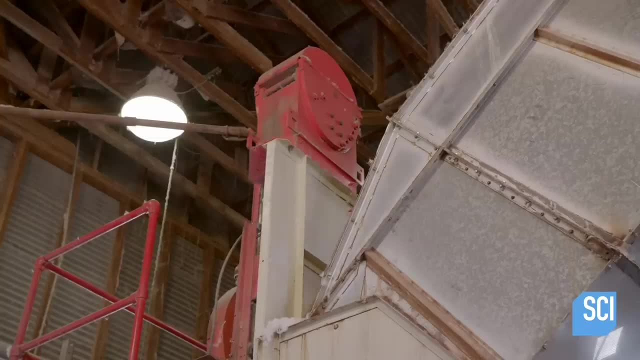 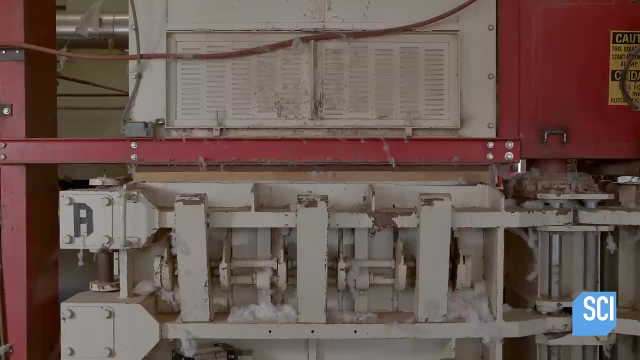 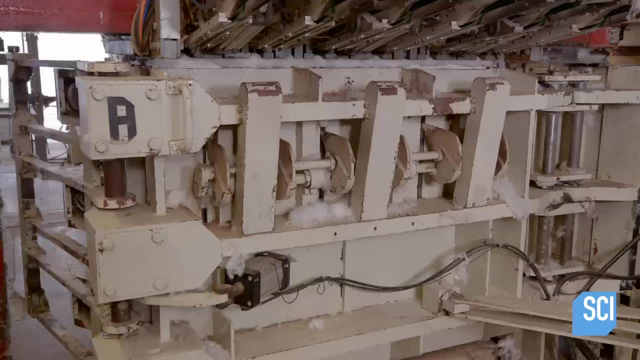 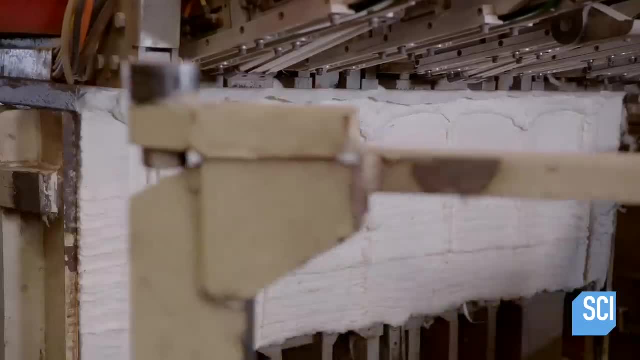 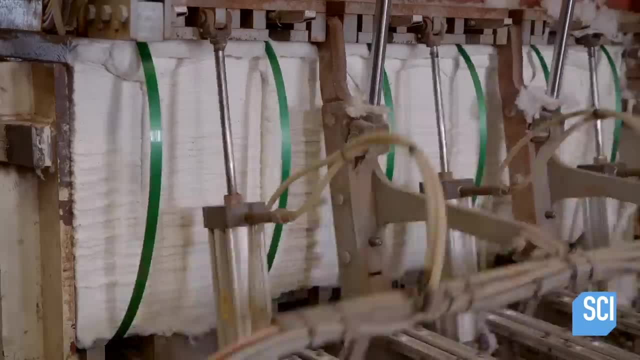 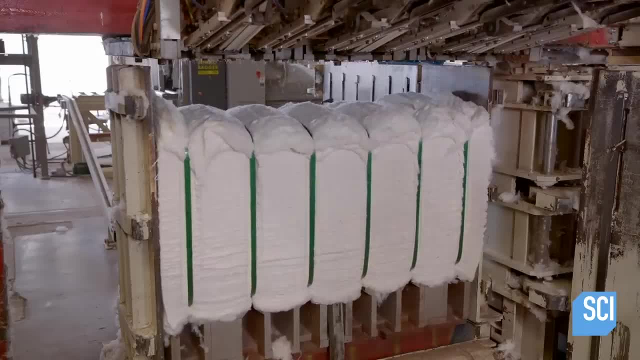 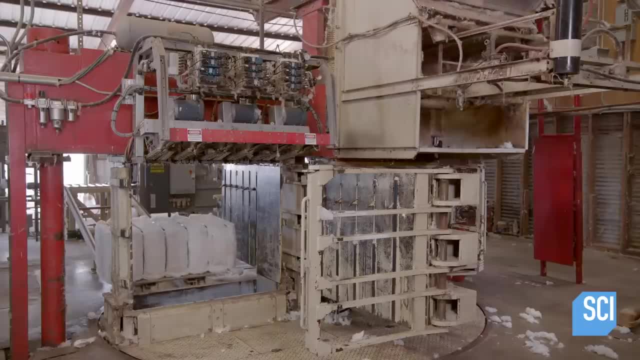 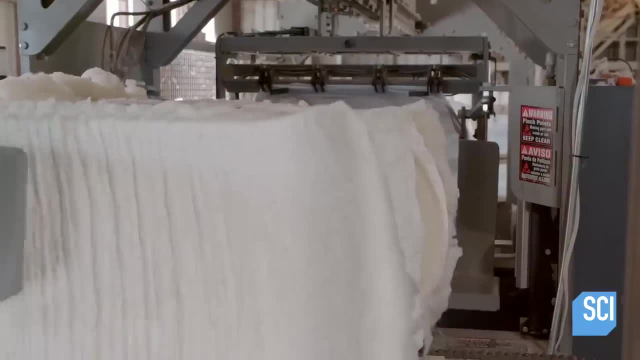 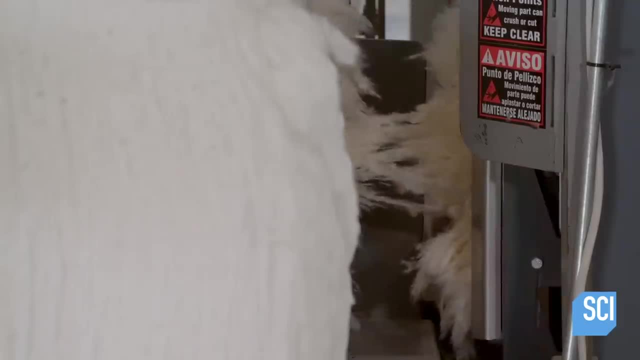 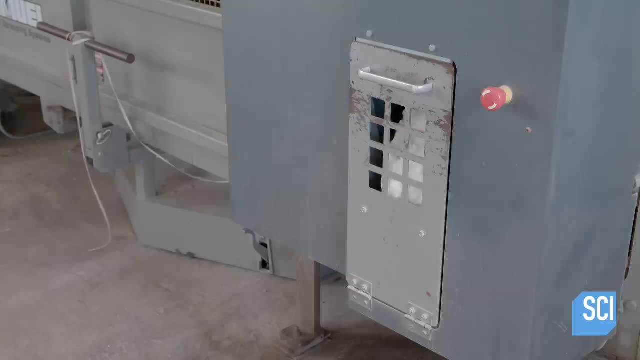 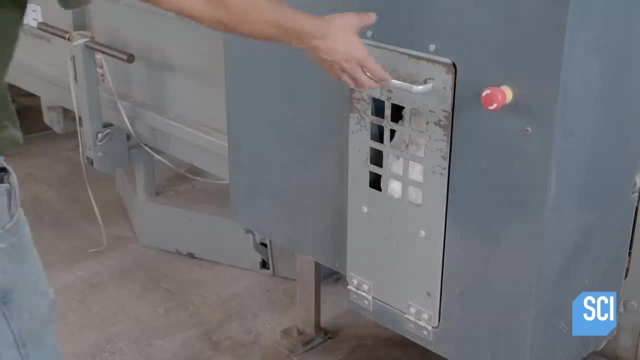 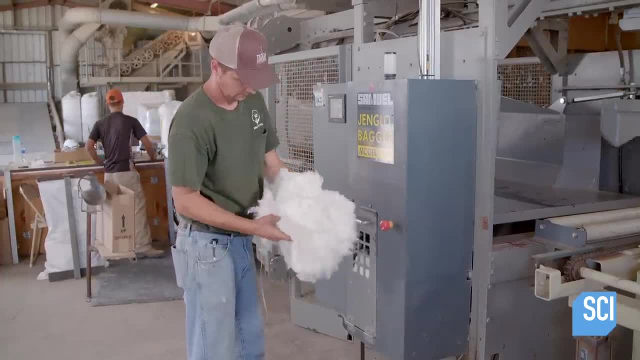 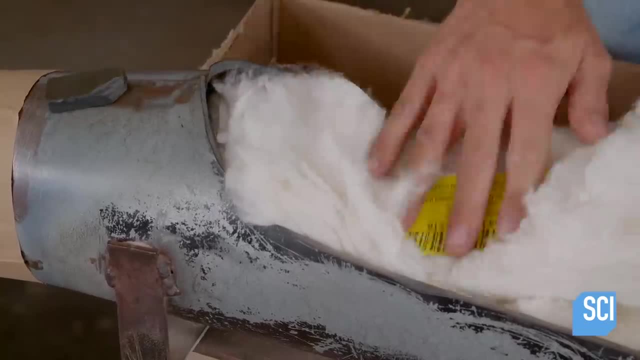 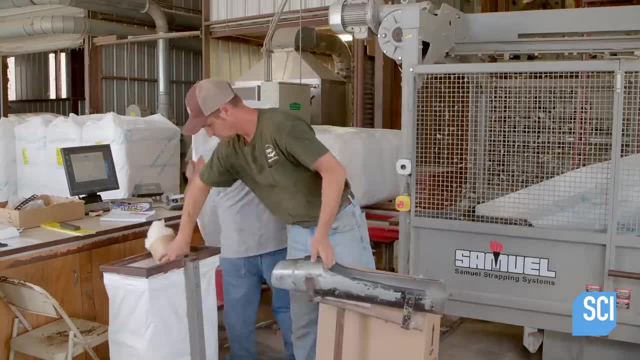 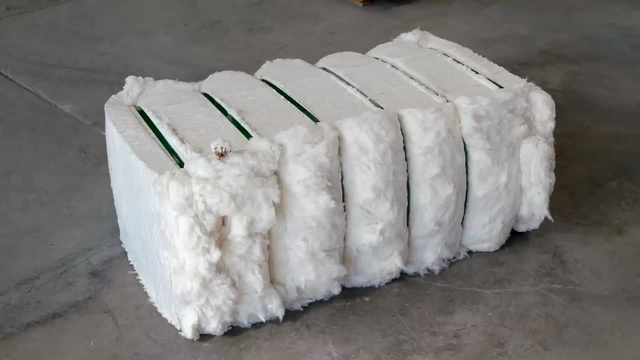